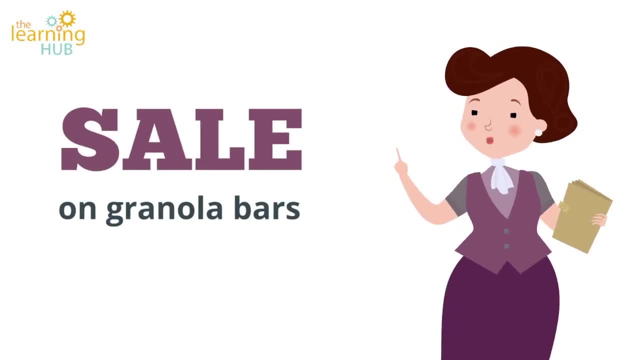 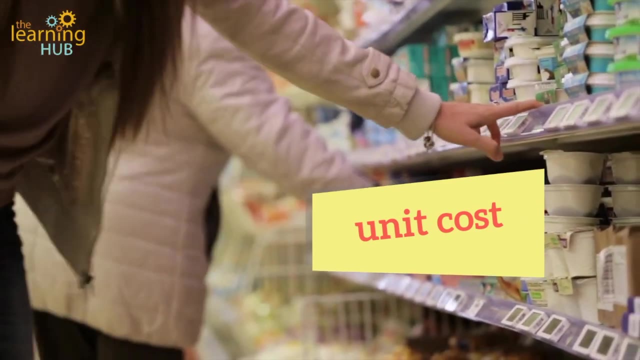 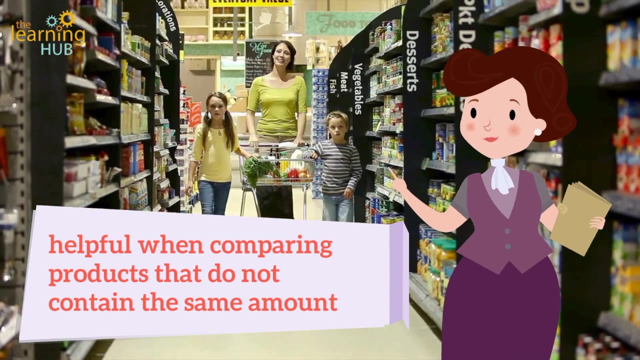 Everybody likes getting a good deal, and getting the best value for your dollar is very important. Math can be really helpful when you are trying to be careful with your money. We can use some simple math calculations to figure out the cheapest product. Finding the unit cost of an item is a great way to find the best value when comparing two products that do not contain the same amount, such as boxes of granola bars. 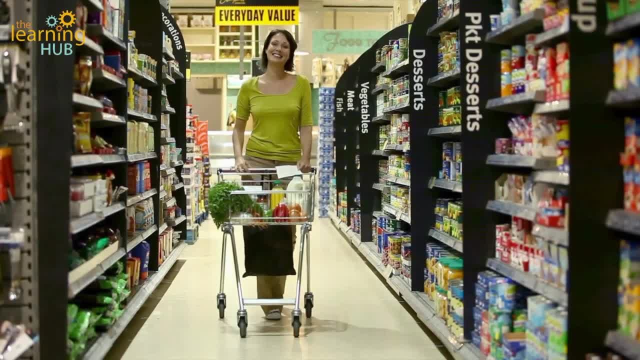 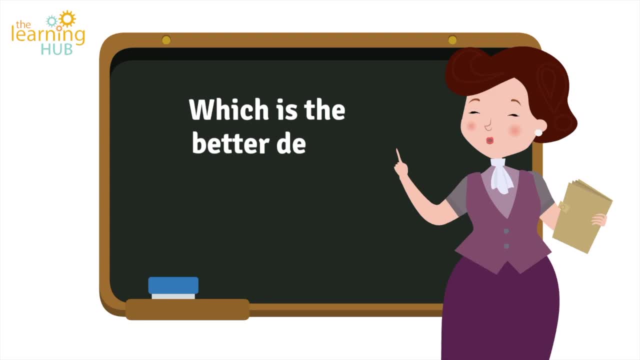 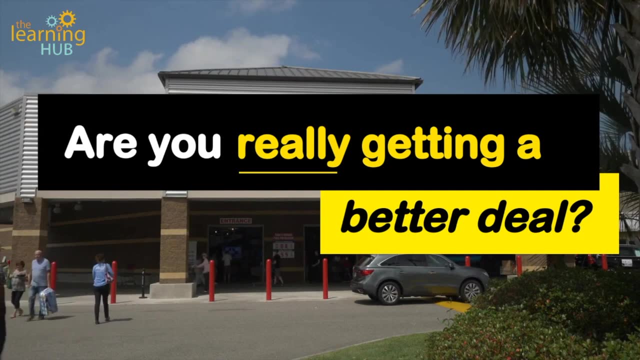 Once you know how much you are paying for a single item in a box, you can compare the two products that contain different amounts. This simple trick is really useful If you like to shop at Costco or other retailers who sell in large quantities. But just because it is a big box store, are you really getting a better deal on your items? 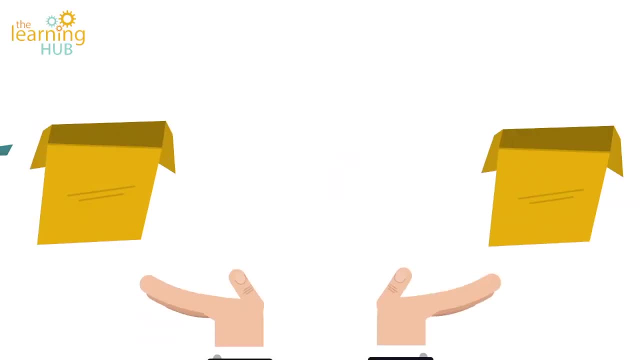 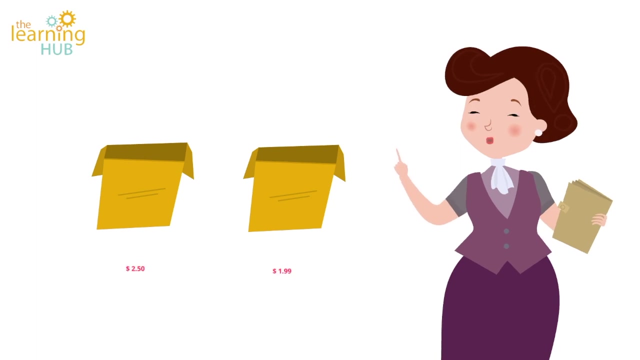 Let's do some comparison shopping. You have two different types of granola bars in your hands. One box of granola bars costs $2.50 and contains six bars. The other box costs $1.99 and contains five bars. Which one is the better deal? 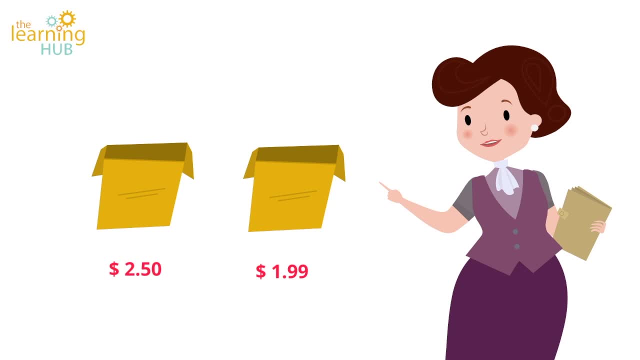 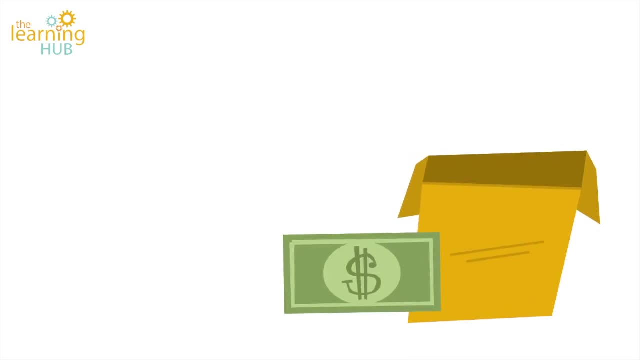 It is difficult to do a quick comparison When the price and number of bars are different. We know that the box that costs less per bar is a better deal. We are going to take the cost of the box and then find out the cost of each bar in the box. 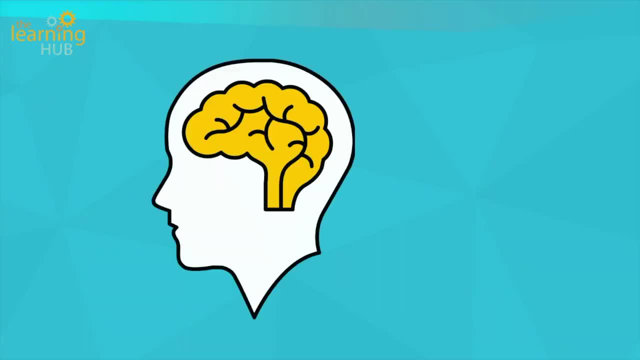 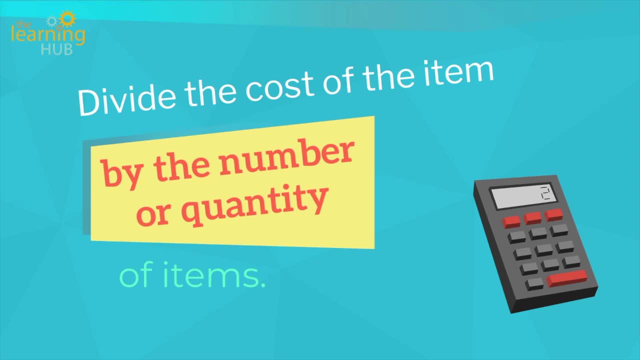 You can use your calculator for this. This is all you have to remember. Divide the cost of the item by number or quantity of items in the box. This works for any measurements such as liters, gallons, ounces. Let's go through an example using granola bars. 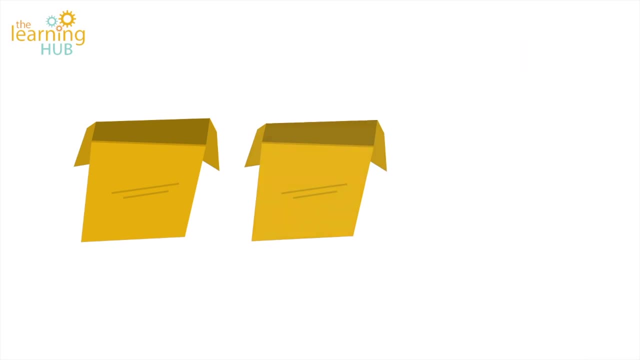 You have two boxes of chocolate granola bars. Box one costs $2.50 and there are six bars. The cost is $2.50 and the quantity is six. Here is the equation you would use in a math class: Cost divided by quantity. 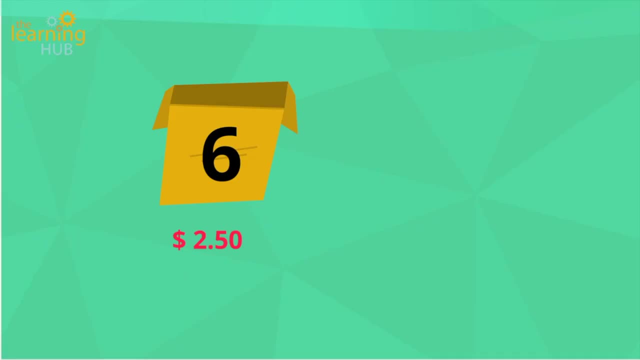 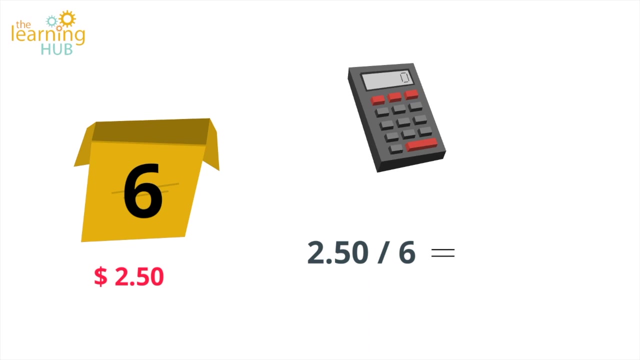 We are now going to substitute the numbers into the equation: $2.50 divided by six. You put the following numbers into your calculator: 2.50 divided by six, This equals 0.41.. What on earth does this mean?